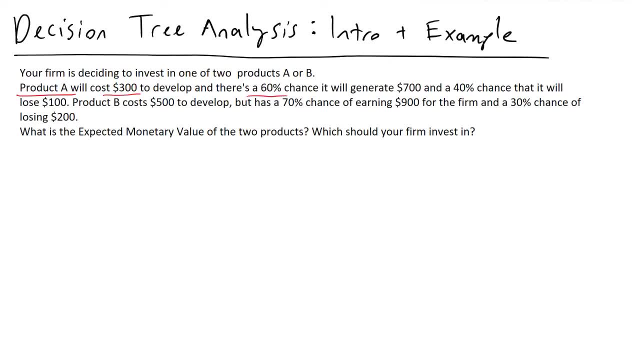 spend $300 to develop it, but our risk analysis have told us that there's a 60% chance that it's going to generate $700 for our company, but a 40% chance that it will lose us $100. And so that's. 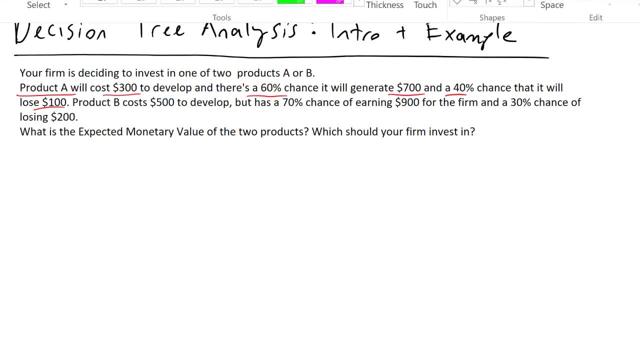 product A. If we go with the path of product B, which I'll use a blue ink to use. if we go with product B, we're going to spend $500 to develop it, but our risk analysis, or analysts, have told us that there's a 70% chance of it making us $900. 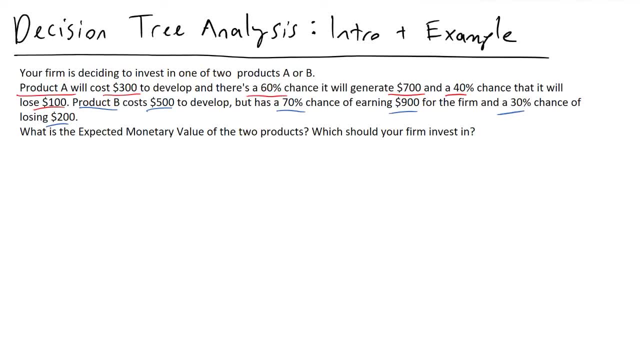 And a 30% chance of it losing $200 for us. And so what our question is is: what is the expected monetary value of these two products? And so that's a new term that we're going to calculate using our decision tree, And the question is: which products should we invest in? Because we're 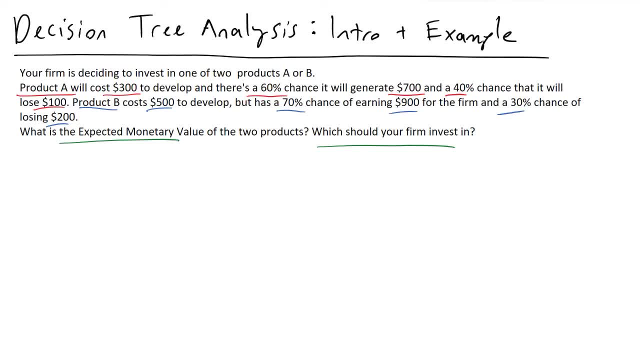 going to only have finite resources and we're going to want to maximize our return on investment for our shareholders. So if you look at the surface of this and you're just like, well, clearly you know we can make $900.. If we go with product B, that looks a lot better than only. 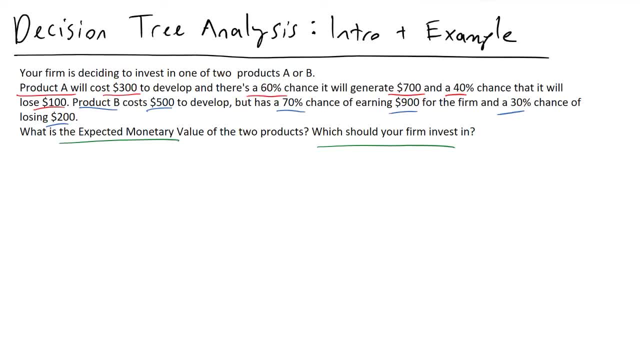 making $700 with product A. Should we really go with product A? And so what we're going to be doing is first just diagramming the situation or the choices that we have. So we've got two choices, We've got product A and product B, And then we also have good and bad situations for each of these. 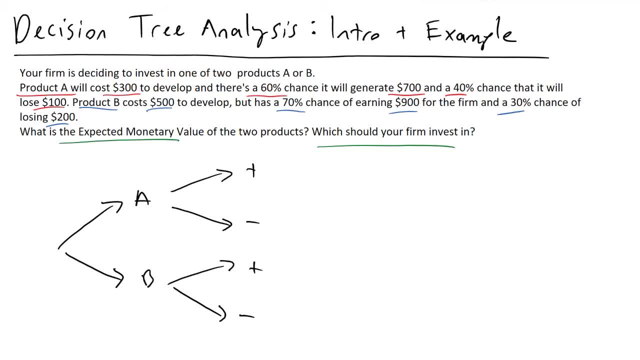 So I'm going to have these two Subsets pointing in either of these scenarios, And so what we know is we begin to fill out. the information that we've been told is that the cost of producing product A is going to be $300. 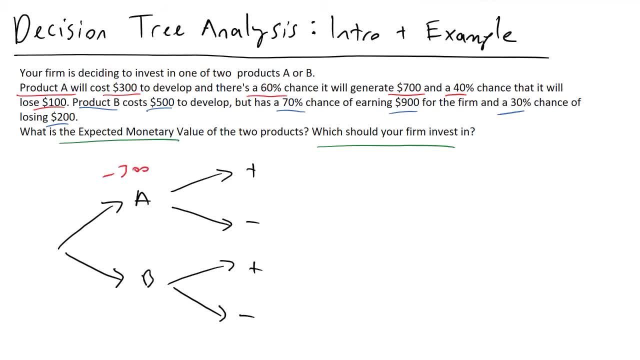 So I'm going to write minus 300 right here And we know that the cost to produce product B is going to be 500. So I will write minus 500 right there In the good scenario for product A. we know that it will. 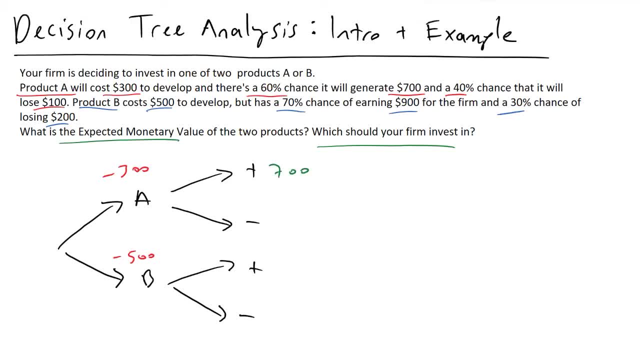 earn us $700. So I'm going to write plus 700 right there, And we know that in the good scenario for product B it's going to earn us $900.. So I'm putting 900 right there And then for the negative, 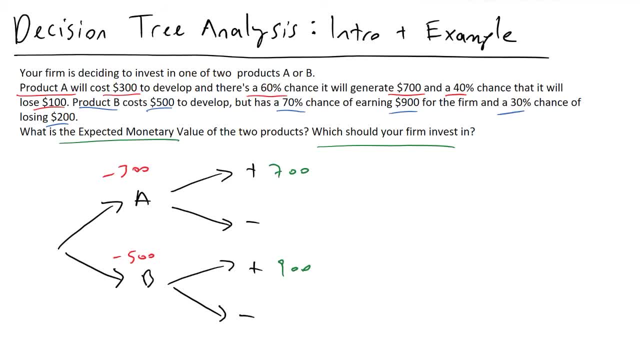 scenarios in which it's losing us money. we know that product A was going to lose us $100. And then we know that product B was going to lose us $200. And now the other thing that we're going to do is we're going to fill in the actual likelihoods of each of these scenarios happening. 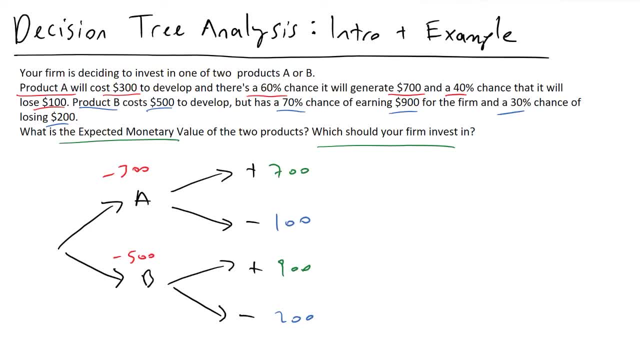 So for product A, our risk analysis told us that there was a 60% chance that it would generate us $700.. So I'm going to write 0.60 right here. And for the bad scenario, that's going to be that 40% chance, So we're going to put a 0.40 right there. For product B, we were told that 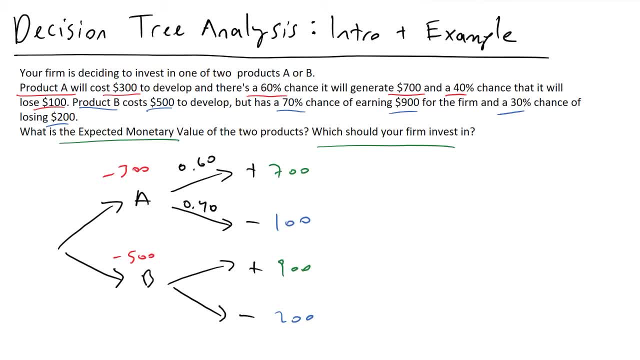 there is a 70% chance of it being the good situation. So I'm going to put a 0.70 right there And we're going to put a 30% chance of us having the bad situation- 0.30.. And obviously this is a 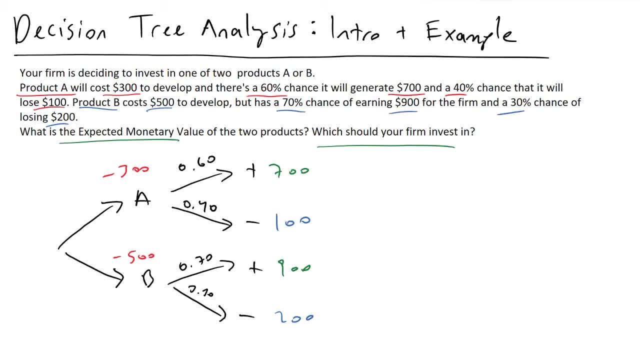 pretty simple example, because we're still learning this stuff, But in the real world there's going to be a ton of other possibilities, And so these things can get a lot more complicated. But, for the sake of getting used to decision trees, this is what we're going to be going with, And so, basically, 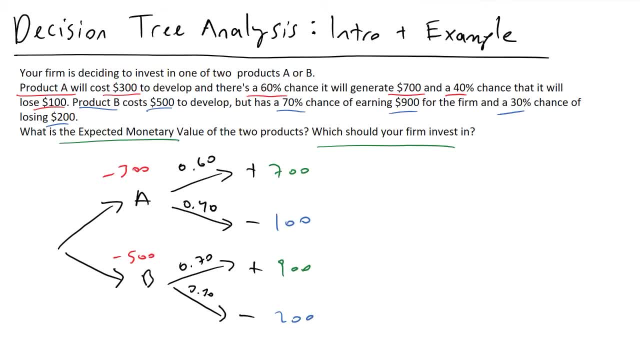 the question that we're trying to answer here is: what is the expected monetary value, EMV, for product A and for product B? So, focusing on product A, what this will be equivalent to- if I was to write this out generically- is we're going to have the development costs of A, which I'll write as d sub a, And then 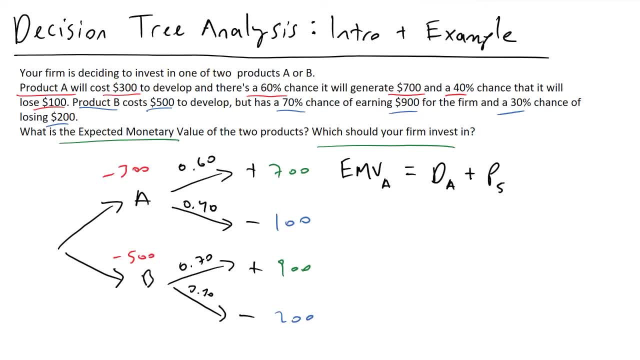 we're going to have the probability of success, which I'll denote p sub s and then times the cost of success, so c sub s. And then we also have the probability of failure, which I'll write p sub f times the cost of that failure, which will be c sub f. 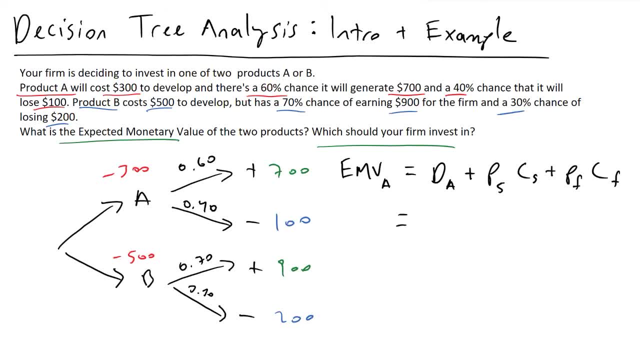 And so if we plug in these numbers, what I'll have is that the development costs of A is going to be minus 300.. And then the probability of success for A was 0.6, or 60%. And then the cost of success. 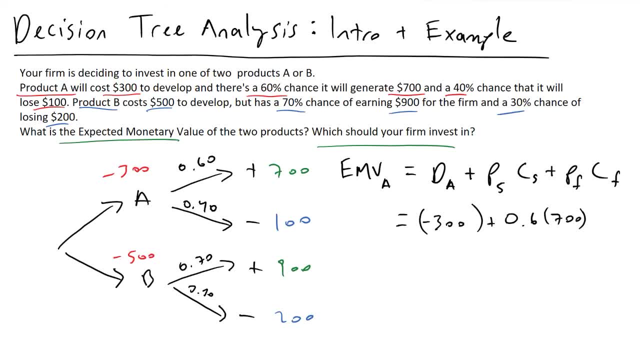 here was $700.. That's positive 700. And then the probability of failure was 0.4.. And then the cost of that failure was minus $100, or that's losing 100 bucks. And so if we plug in these numbers, we'll have the. 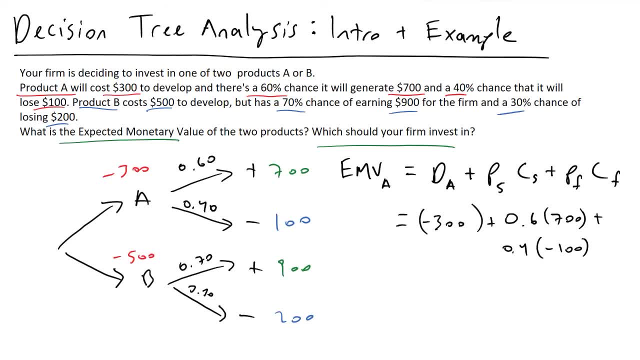 problem that we're going to get $1,000. And then we're going to end up getting $80. And so for that, what we're going to find is that we end up getting $80.. If we were to add up all these numbers, 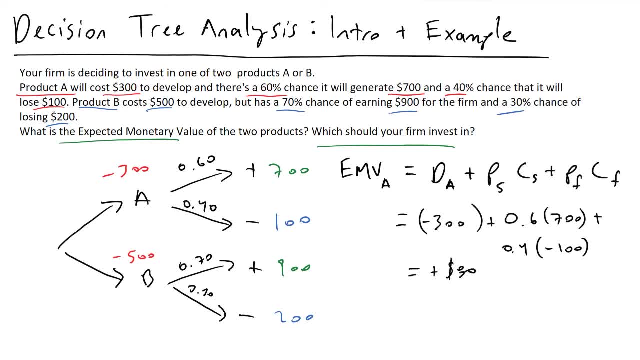 what we are going to find is that we end up getting 80, plus 80. And we'll just try to write that clearly. And so what this number is telling us is that, for product A, if we were to make infinitely many decisions and go with product A on every single one, on average, this would be an infinite number. 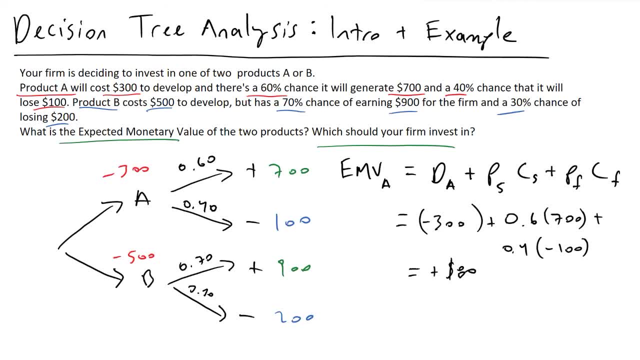 be netting us 80 dollars in return for our choice. so that's what we know about product a. now, if we go with product b, which i will denote as emv, sub b, the expected monetary value of b- this will be equivalent to that minus 500 bucks that we spent developing it, plus the 70 chance that it got us. 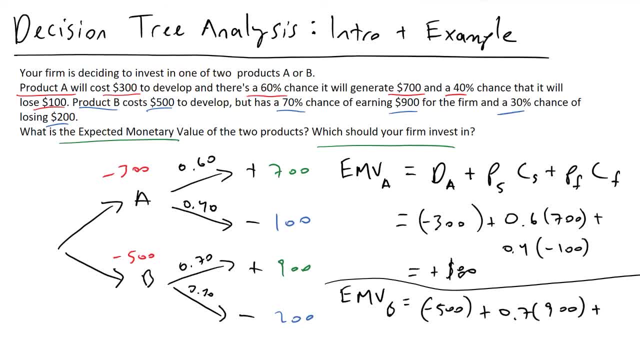 900 bucks, and then plus the 30 chance that it got us that loss of 200 bucks, and this number is equal to plus 70 or 70 dollars. and so what this tells us is that when we look at the expected monetary values for both a and b now, is that product a in the long run will actually be. 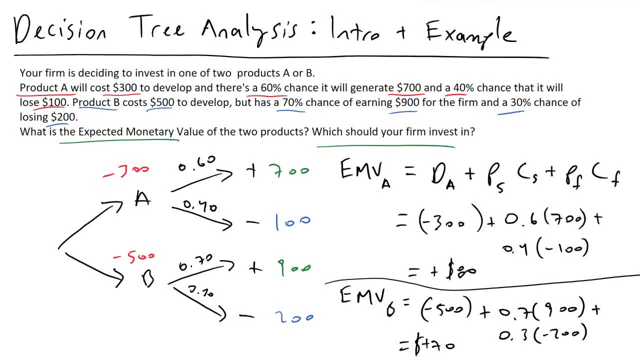 returning us a higher profit or return on investment than product b, and so that is the reason why we know that product a is going to be a higher return on investment than product b, reasoning why we went through this whole decision tree analysis, looking at both the positive and 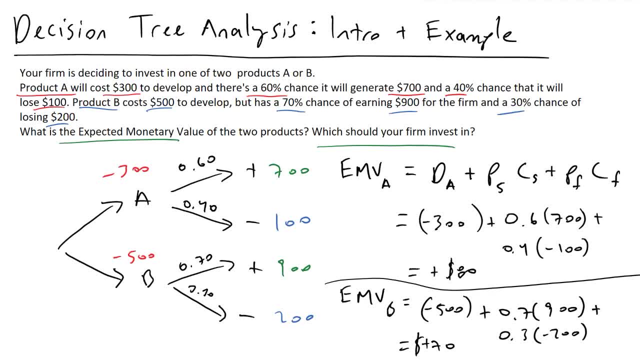 negative scenarios for both of these products in our decision, and so the conclusion that we're coming to is that, because the expected monetary value of a is higher, if we had finite resources and we could only make one choice, our firm should move ahead with focusing on developing and. 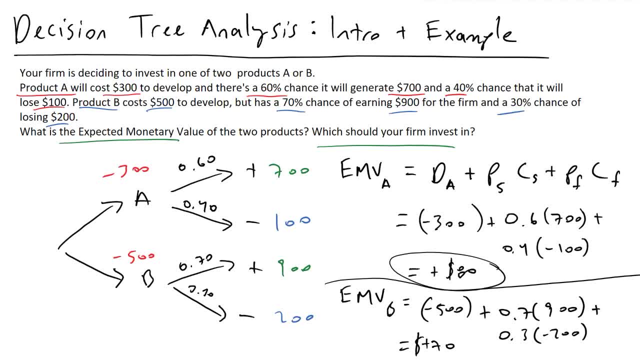 selling product, a. so that's going to wrap things up for this video. i hope it helps, let me know if you guys have any questions, and thank you all for watching.